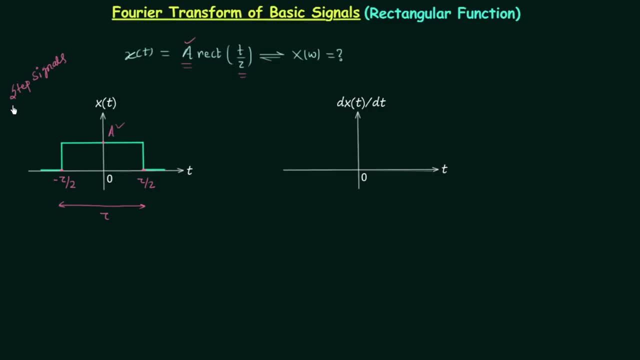 of step signals and therefore for the calculation of Fourier transform we can use the method of differentiation. We will differentiate the signal waveform and from the obtained result we will calculate the Fourier transform. So let's quickly perform the differentiation of the given waveform. For this we will start from minus infinity and you can see from minus infinity to minus. 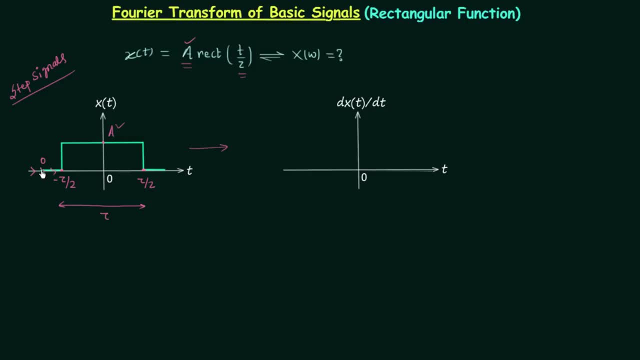 tau by 2, the signal value is equal to zero and it is constant. So the waveform of signal dxd over dt will have the value equal to zero, from minus infinity to minus tau by 2, because this will give us the slope of signal xt and the slope of this. 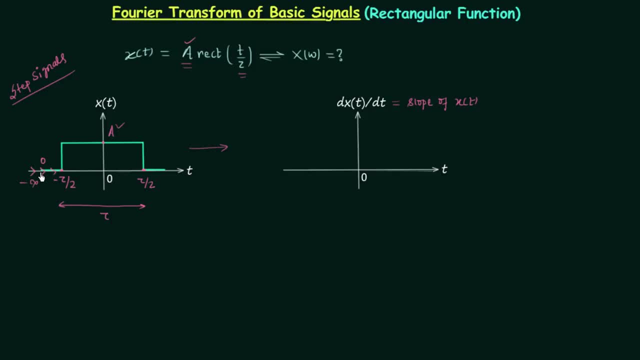 line from minus infinity to minus tau by 2 is equal to zero. Let's say: this instant here is minus infinity Minus tau by 2 and this instant here is equal to tau by 2.. So we have value of signal dxd over dt equal to zero from minus infinity to minus tau by. 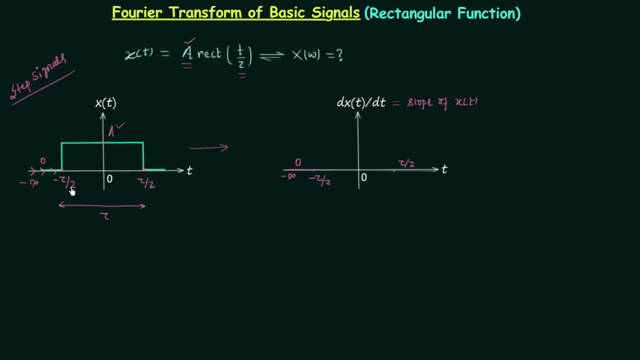 2, and after this, when t is equal to minus tau by 2, xt is having the upward level switching, So we have the infinite value of the slope. So dxd over dt will be zero. So the wave of the signal is represented by an impulse and the weight of this impulse. 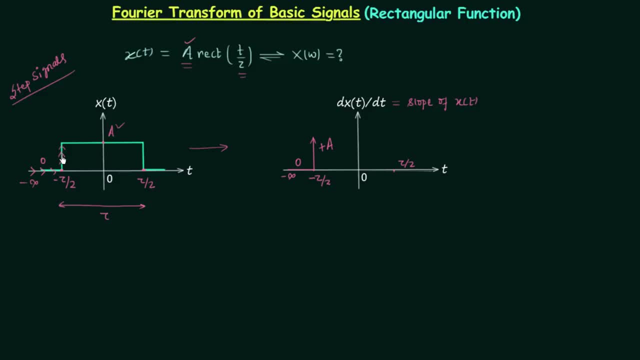 signal is equal to plus a. We are having plus because there is upward level switching and we are having a because the discontinuity is equal to a. Here the value of signal is equal to zero and here the value of signal is equal to a. 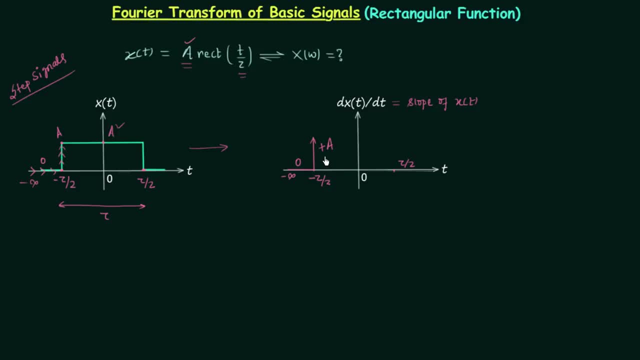 So a minus zero will give us the discontinuity which is equal to a plus a. Now we will move forward and you can see the value of signal is equal to a from minus tau by 2 to tau by 2, and this line is having the slope equal to 0.. So dxd over dt. 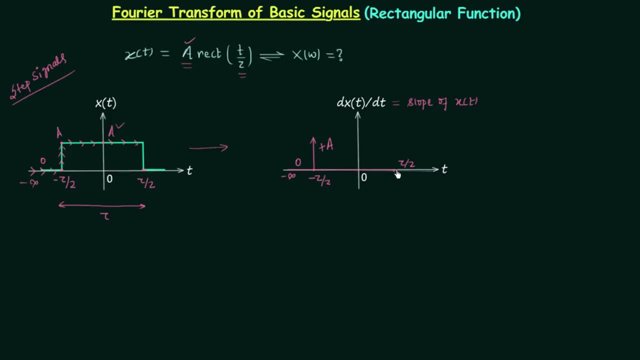 will be equal to 0, from minus tau by 2 to tau by 2.. After this we are having downward level switching and again the discontinuity is equal to a, and as it is downward level switching, the weight of the impulse will be negative. So we will have the impulse like 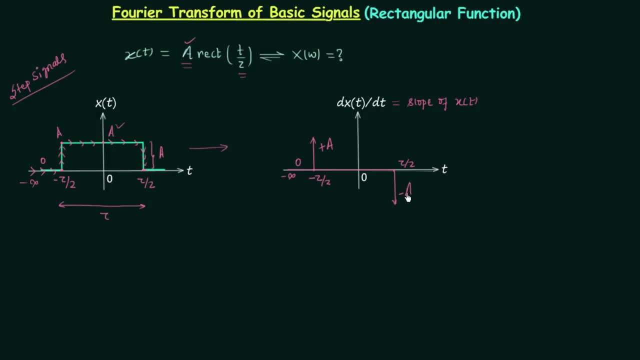 this and it is having the weight minus a. After this we are having xt equal to zero, from tau by 2 to plus infinity, and you can see this line is having the slope equal to zero. So dxT over dt is equal to zero, from tau by two to plus infinity, and in this way we 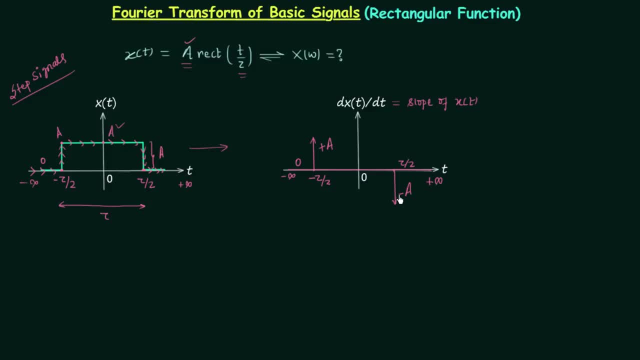 have the signal, which is the combination of only impulses. Therefore we can calculate the Fourier transform of rectangular function easily using this waveform. So let's quickly represent the signal dxT over dt in terms of impulses. There are two impulses and the first impulse is equal to a deltaT plus tau by two, and the 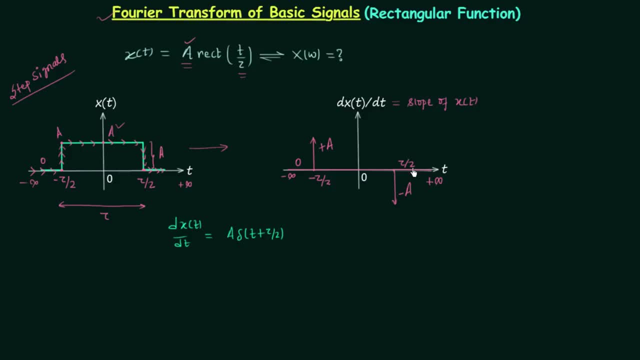 second impulse is equal to minus a deltaT minus tau by two. I will take a common. So dxT over dt is equal to a Bracket Bracket deltaT plus tau by two, minus deltaT minus tau by two. Now we will perform the Fourier transform on both the sides. 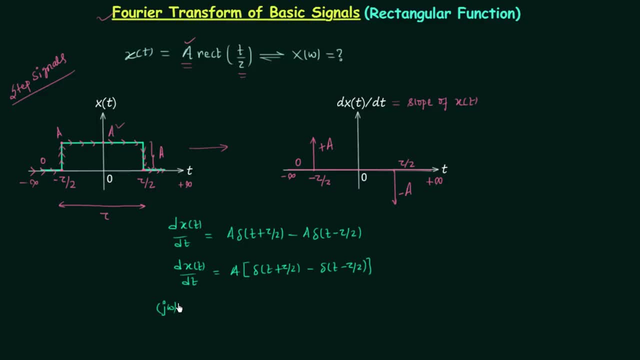 On the left hand side we will have j omega power one multiplied to x omega, where x omega is the Fourier transform of signal xt. On the right hand side we will have a bracket, Fourier transform of deltaT plus tau by two. Fourier transform of deltaT is equal to one, but here we are having deltaT plus tau by 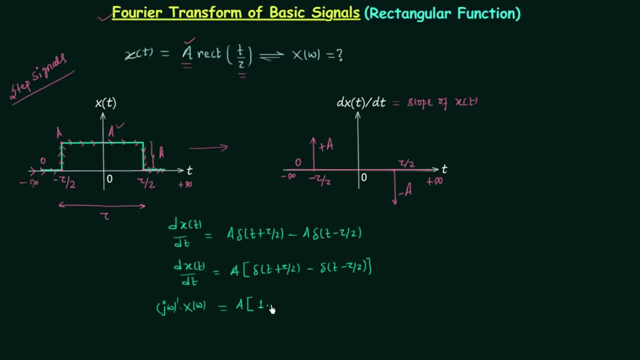 two. So we will use the property of time shifting and this one will be multiplied by e power, j omega tau by two. Similarly, from here we will have one multiplied to e power minus j omega tau by two. So we have j omega multiplied to x omega equal to a. 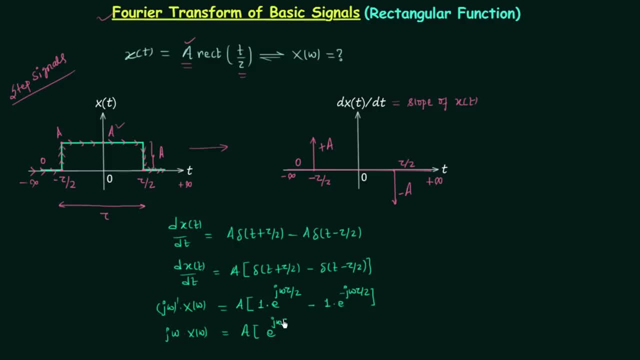 Inside the bracket: e power- j omega tau by two minus e power minus j omega tau by two. And now we will divide both the sides by j omega. So we will have x omega on the left hand side and on the right hand side we will have a. 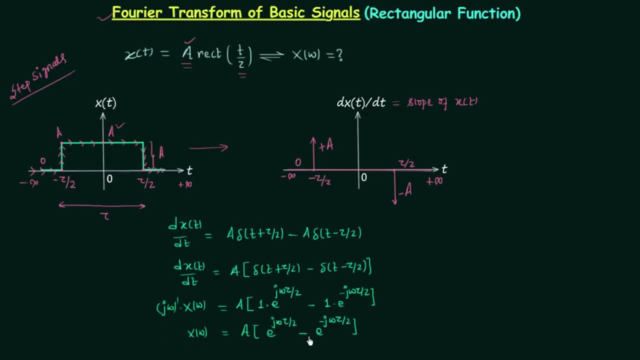 multiplied to e power j omega tau by two minus e power minus j omega tau by two, divided by j omega, We can write: e power j omega tau by two minus e power minus j omega tau by two, divided by j equal to two times sine omega tau by two. 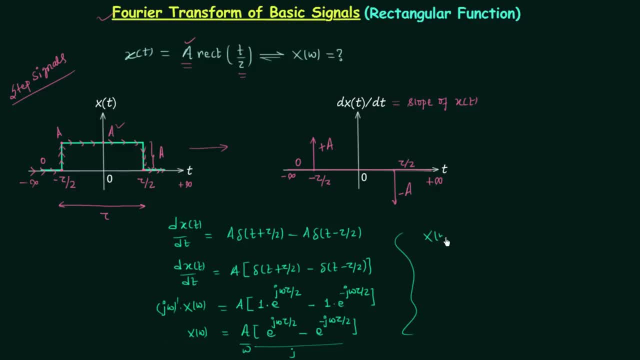 So we will have x omega equal to a over omega, multiplied to two times sine omega tau by two. Now I want to write x omega, I want to write x omega in terms of sampling function, therefore, I will divide by omega tau by two and multiply by omega tau by two. 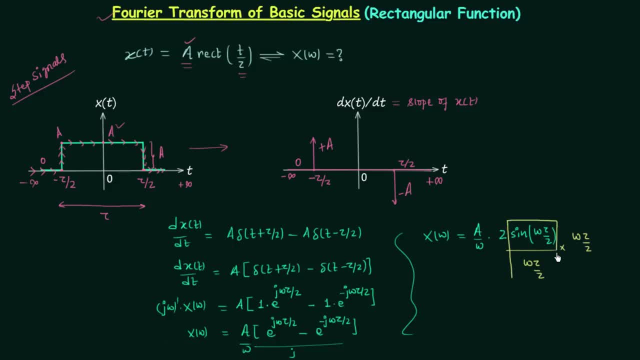 So sine omega tau by two, divided by omega tau by two is equal to sampling omega tau by two. So we can write Fourier transform x omega equal to j omega tau by two. So this is the Fourier transform x omega equal to a, because this omega and omega will cancel. 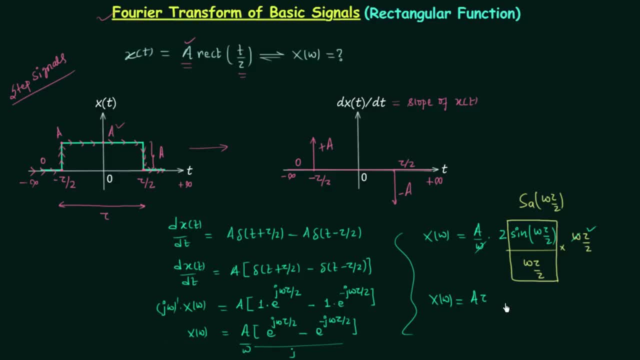 out multiplied to tau, this tau here, sampling omega tau by two, This two and two will also cancel out. So this is the final result. You have to remember this Fourier transform. This is the Fourier transform of rectangular function. And now you will ask me: 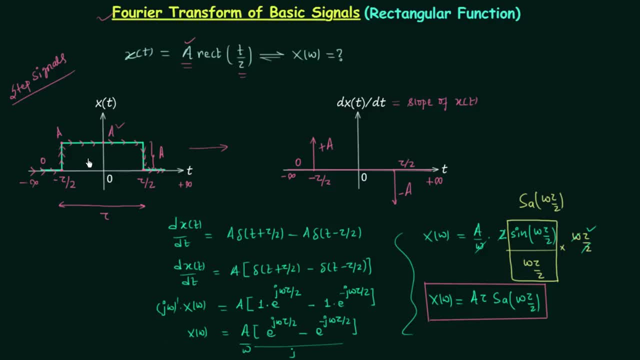 What about the dc value? The dc value of this signal is equal to zero because this signal is finite duration signal and finite duration signals have dc value equal to zero. The dc value is equal to zero because xt is non-zero for a very small amount of time.